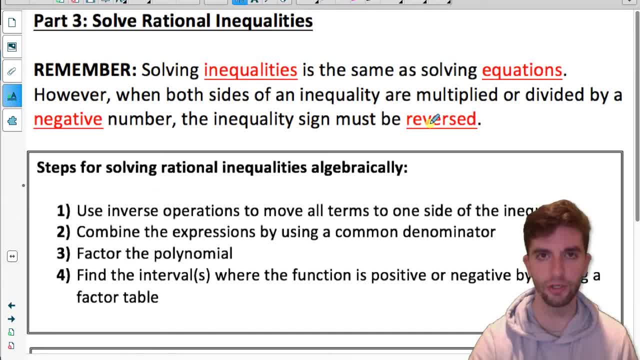 inequalities from when we solved polynomial inequalities earlier in the course. So we learned when solving polynomial inequalities that we could solve them just like equations, as long as we followed one rule: when both sides of the inequality are multiplied or divided by a negative number, we had to reverse the inequality sign. So that was an easy rule to follow. if we were solving a linear inequality, that was fine. But if we got higher degree inequalities like degree two, degree three or so on, we figured out we might. 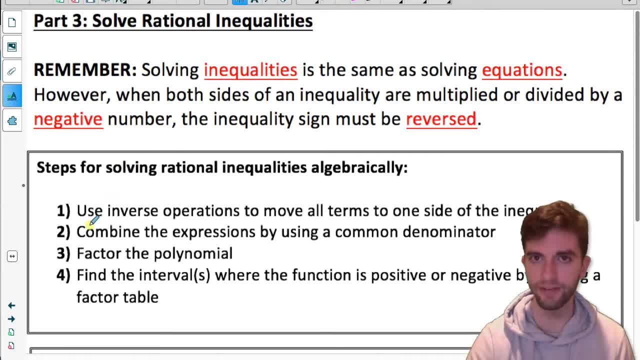 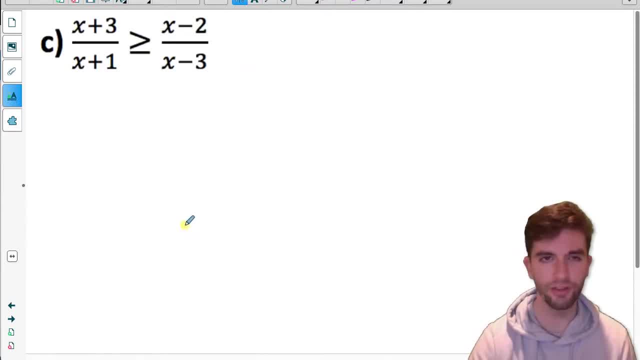 be easier to solve them if we solve them graphically or by making a factor table. So what are we going to do for these types of inequalities? Well, we're not going to try and solve these algebraically, like equations, and then try and follow that rule of reversing the inequality when we multiply or divide by a negative. We're not going to do that Because if I multiplied both sides of this inequality by x plus one and x minus three to try and get rid of the fractions, do I have to reverse the inequality? Did you just multiply by a negative? if we're 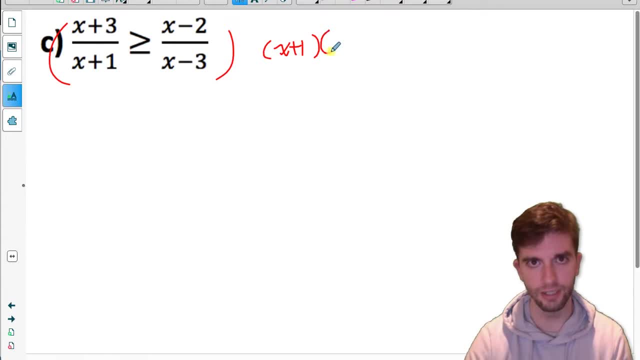 multiplying both sides of this by x plus one times x minus three. Well, is x plus one negative Sometimes depends on the value of x, And is this negative Sometimes? So it depends on the value of x. So we would have to split our algebraic solution into different cases Depending on the value of x. we might have to reverse the inequality And the process gets pretty complicated pretty quick. So we're not going to solve it algebraically, So maybe we'll solve it graphically. We 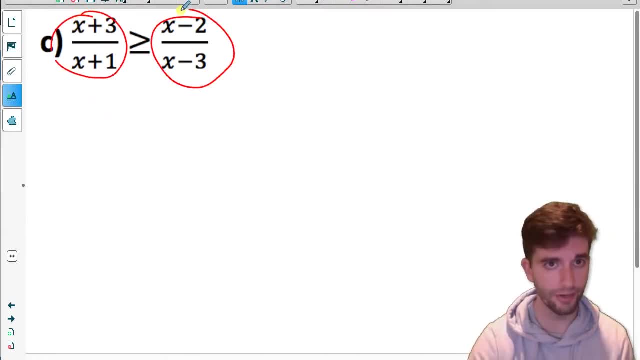 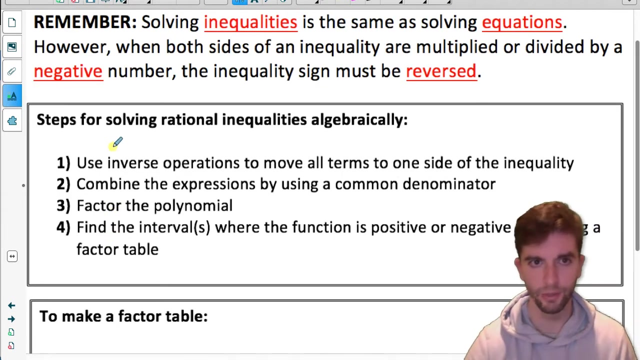 could. we could figure out what the graph of this looks like in the graph of this looks like and then figure out when is the one on the left greater than the one on the right? But that would be fairly complicated as well to generate those graphs and get exact values where we know that the one on the left is greater than or equal to the one on the right. So I think the most efficient thing to do is to make a factor table. So let's go over how we're going to make a factor table. So, before we make the factor table, we're going to follow these steps. We're going to start by moving all of the terms to one side. 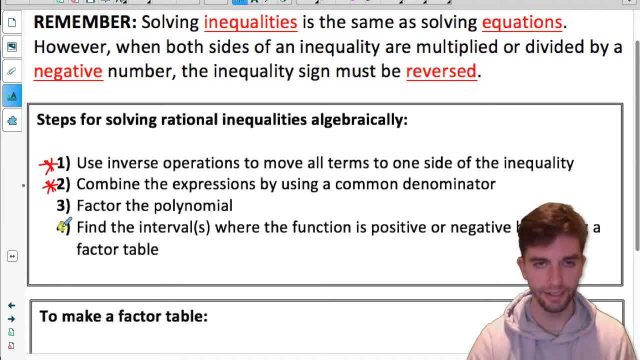 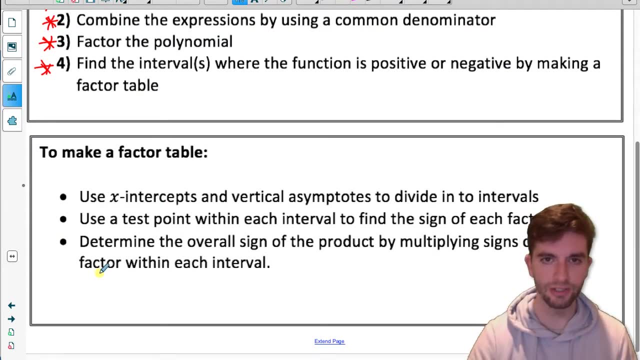 After we do that, we're going to combine the terms by getting a common denominator And then we're going to factor everything as much as possible And then make our factor table, sometimes also called a sign chart. And how do we make a factor table? I'll reference these steps as we actually do the questions, But I'll just go over them quickly now. In the factor table we use the x intercepts and vertical asymptotes. I'll explain why in a little bit, as our dividing points. 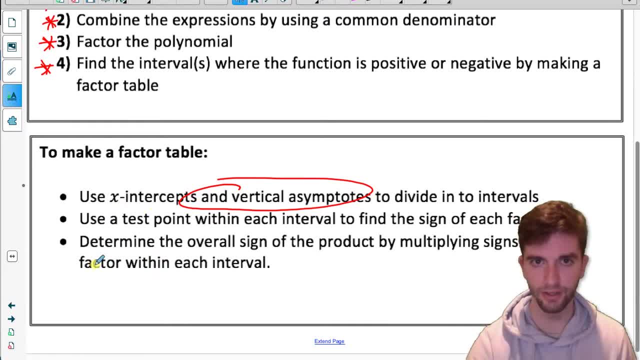 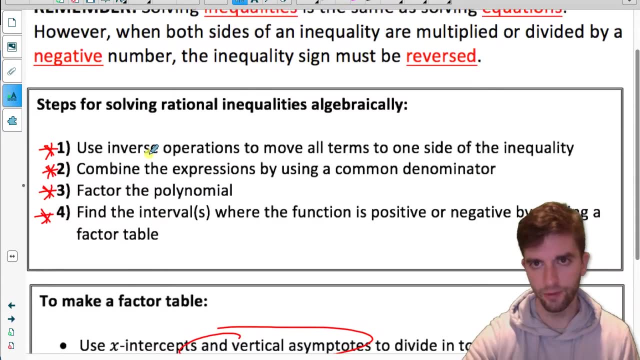 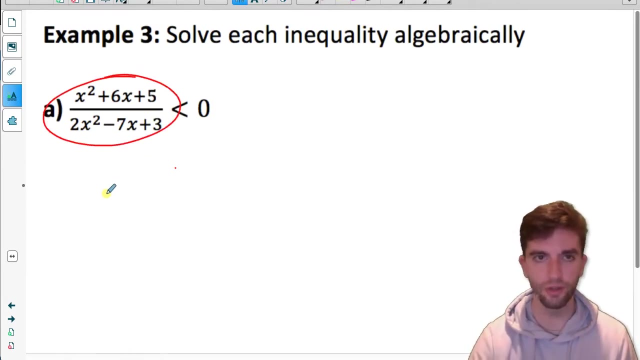 And then we choose a test point within each interval between the x intercepts and vertical asymptotes, And then we plug those test points into all the factors of the polynomial and inequality to see whether it's positive or negative And that'll tell us whether it's greater than or less than zero within each interval. So those steps may seem a little bit overwhelming, just me reading them over, But let's give a question a shot and see how they work. So this first one- all of the terms are already moved to the left. on the right side of the inequality is just zero. So step one is done, everything's already moved to the left. 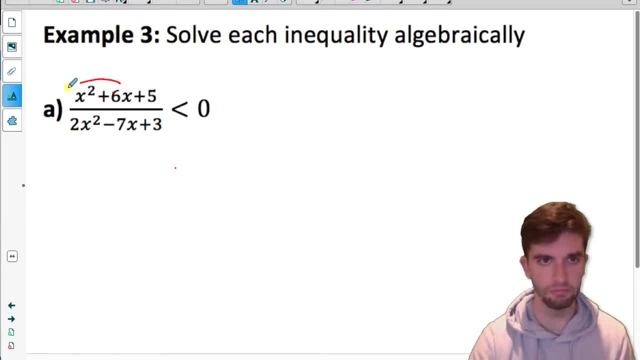 over. Step two says: combine everything and write it as a single fraction. Well, this is already written as a single fraction, already done for us. So the first two steps of this one are already done. Step three is factor it So in the numerator. I have a quadratic where the a value is one, so I 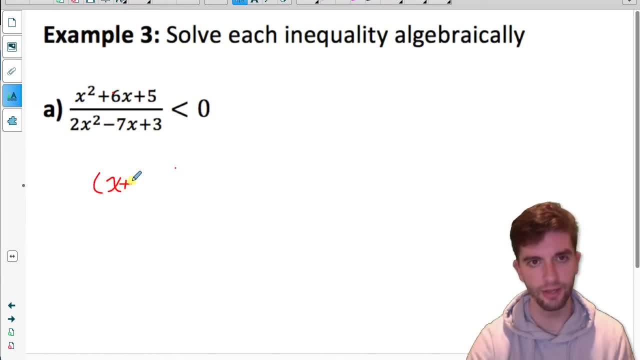 can just find a product of five and a sum of six, and that's x plus five times x plus one. In the denominator the quadratic has an, a value that is not one. so I would have to find two numbers that have a product of a times c, so a product of six and a sum of negative seven and those two numbers 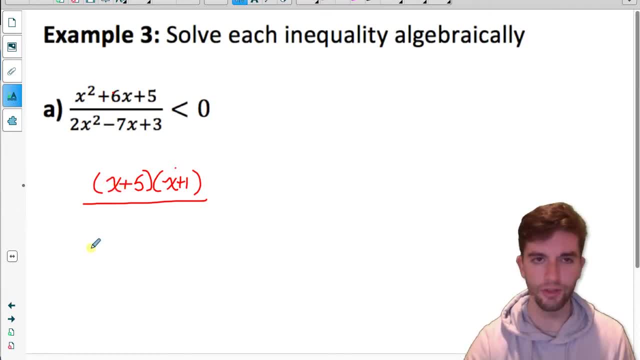 are negative six and negative one. Now there's a bunch of shortcuts to use those numbers to come up with the factors, but I'm just going to off to the side, do it the long way by decomposition. Okay, now that I've figured out the factors, I can write them over here. It's x minus three. 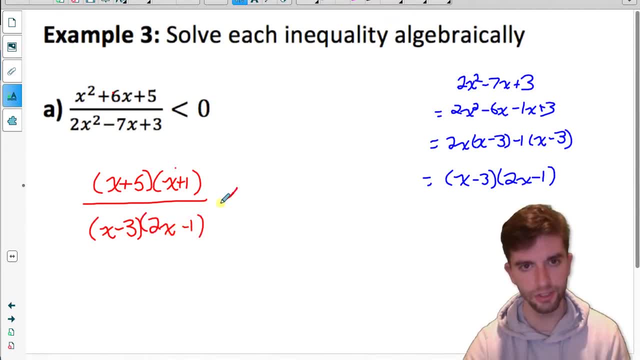 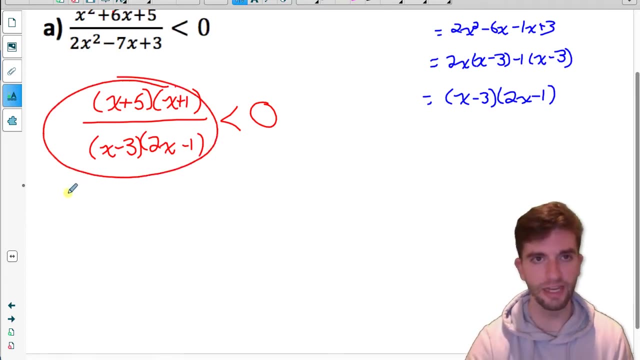 times two x minus one, And I'm interested in when? is this less than zero? So you might be wondering: okay, well, why did we bother factoring this? Well, it's important to get this factored because from the factored form version of this polynomial I could figure out where this function's x-intercepts and vertical. 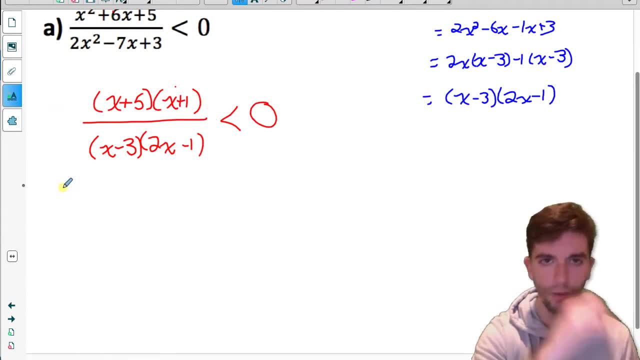 asymptotes are, and those are going to be the important points of this function. to help me figure out when it is going to be less than zero, Let me start by finding the x-intercepts and vertical asymptotes and then show you a graph of this and hopefully you'll be able to. 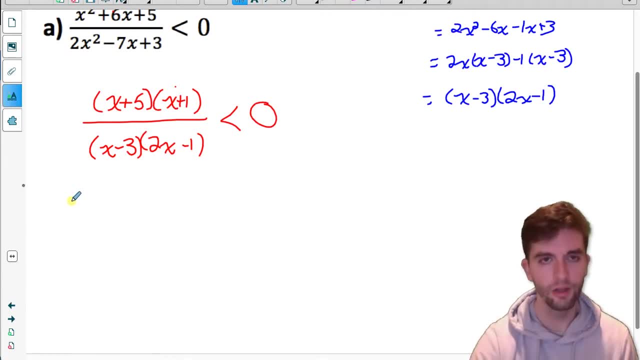 make the connection as to why we're finding them. So an x-intercept is an x value that would make the y value be zero. So what value of x would make this whole thing become zero? Well, what makes a fraction be zero is if the numerator is zero. So how could the numerator of this be zero? So the 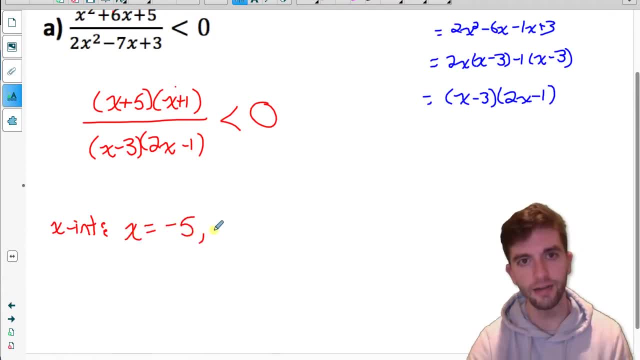 x-intercepts are at x values of negative five and negative one. And where are the vertical asymptotes of a function? The vertical asymptotes are at x values of negative five and negative one. So what would make the denominator of this become zero? X cannot be three or a half, So I have two. 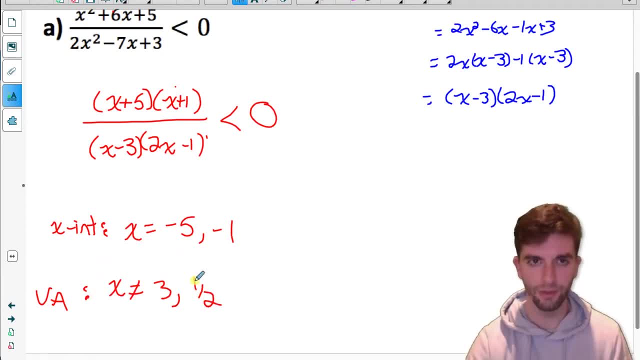 vertical asymptotes They would be at x equals three and x equals a half, because those two values make the denominator of this become zero, which means this whole rational function would be undefined. So now that I have the x-intercepts and the vertical asymptotes, I can actually 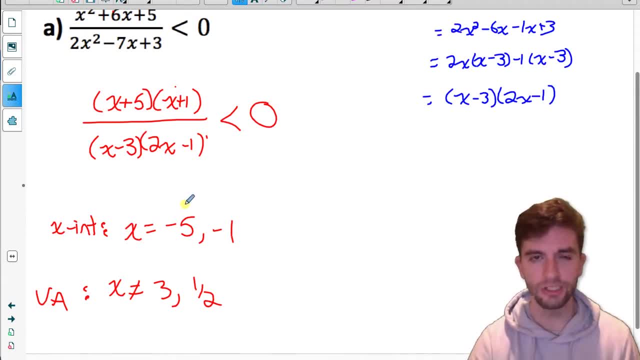 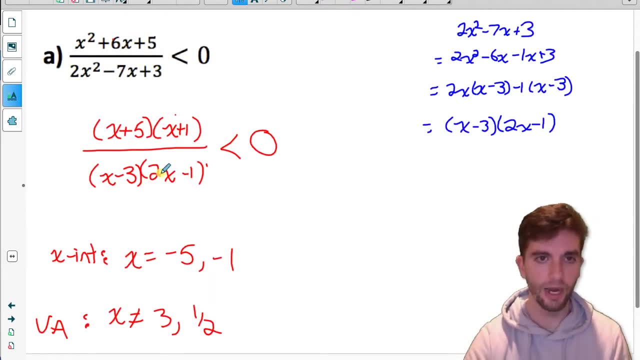 figure out when the function is going to be less than zero by carefully choosing some test points and setting them up in a factor table. Let me actually backtrack a bit and show you the graph of this, so you can hopefully understand why we're doing. 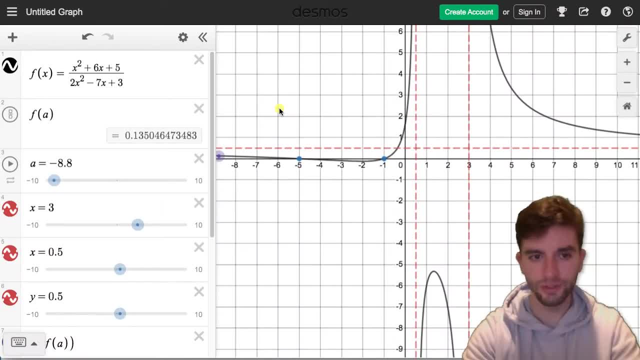 this process. So here's the graph of the function We're interested in. when is this function less than zero? That's what our original inequality says. It says when is it less than zero? So, looking at the graph we're looking for, when is the function below the x-axis? When does it? 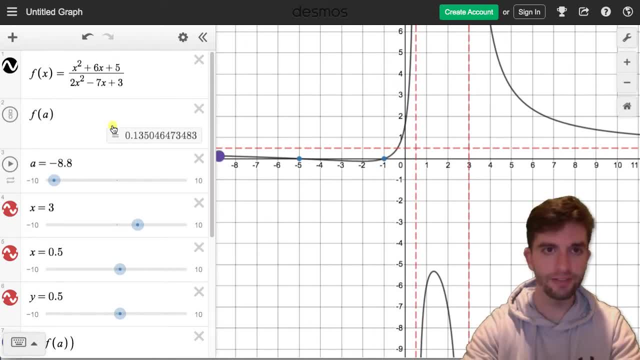 have negative y values. Well, I have Desmos calculating the y values for me for any value of x. So I'm going to go ahead and do that. So I'm going to go ahead and do that value of x and I'm just going to drag this purple point along so you can see at that purple. 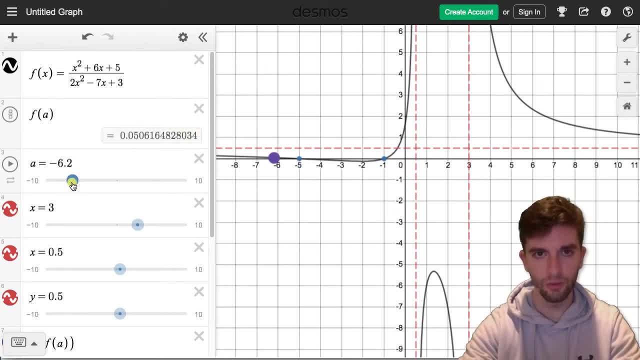 point. it's calculating the y value for me. So before the x-intercept of negative five, notice all those y values are positive. But after the x-intercept of negative five the y values become negative. So at the x-intercept of negative five the function switched from being positive before. 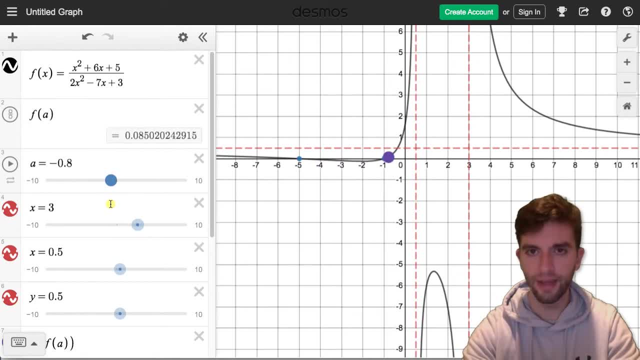 to being negative after, And then at the x-intercept of negative one is the place where it switches back from being negative before to positive after. So it's easy to see that of course, at an x-intercept that's a place where a function might switch from being positive to. 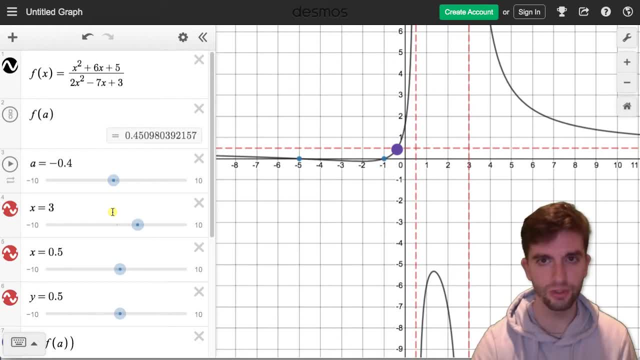 negative or vice versa. So x-intercepts are crucial, dividing points that we might want to test between, to see if the function is positive or negative, to see if that interval is an answer to our inequality. We're looking for intervals that output values that are less than zero. So right, 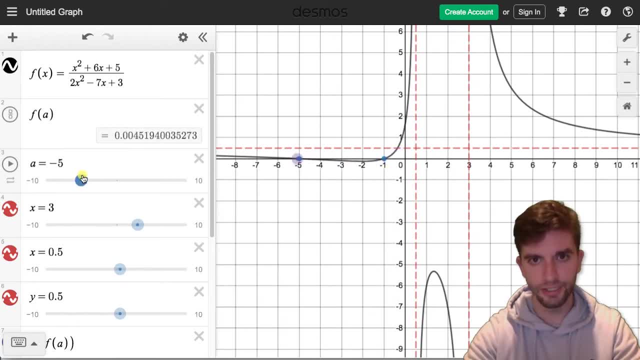 now, based on what we've looked at so far, the interval between the x-intercept of negative five and negative one is a solution to our inequality. Any x-value between negative five and negative one yields a negative y value, So a value less than zero. But the function can also switch from being 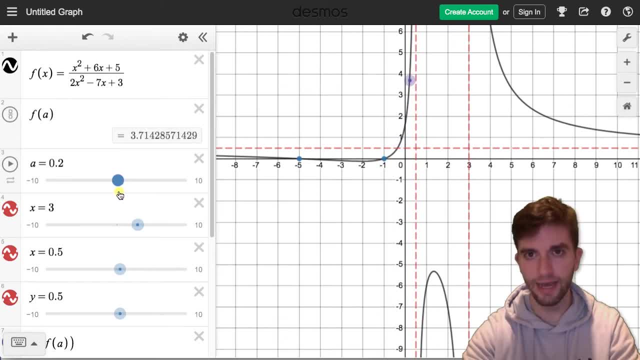 positive to negative around vertical asymptotes. right After the vertical asymptote of half, the function jumps way down here to this other part. So it was positive y values up here After the vertical asymptote, it jumped way down here And now it has. 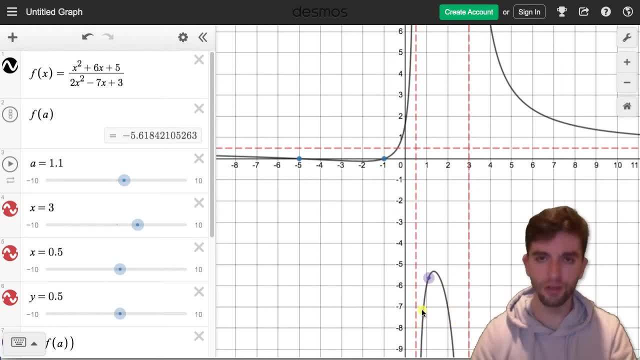 negative y values. So vertical asymptotes are other important dividing points where the function could switch from being positive to negative or vice versa, And then, once it gets to the next vertical asymptote, at an x value of three, it jumps back up to being above here where the y 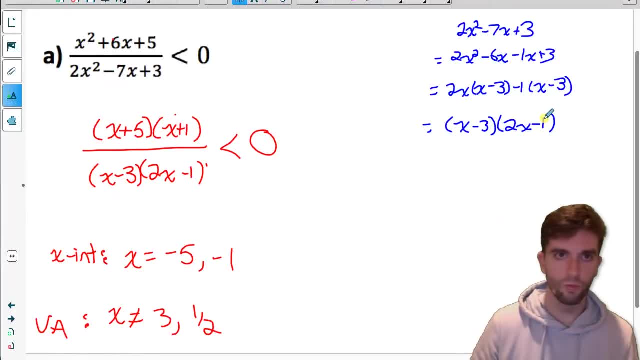 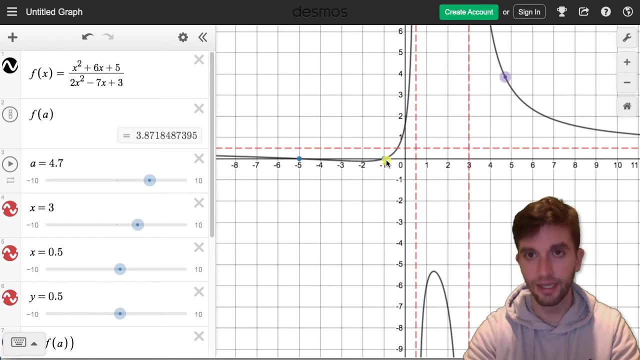 values appear positive again. So we're looking for when is the function less than zero? If we have the graph, we can see it's between negative five and negative one, and also again between a half and three. So there are two intervals where the function is less than zero. How are we going? 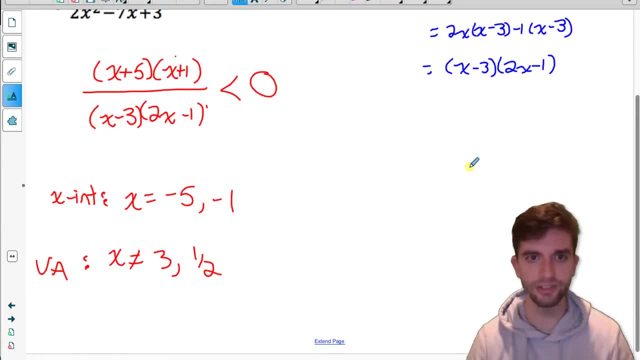 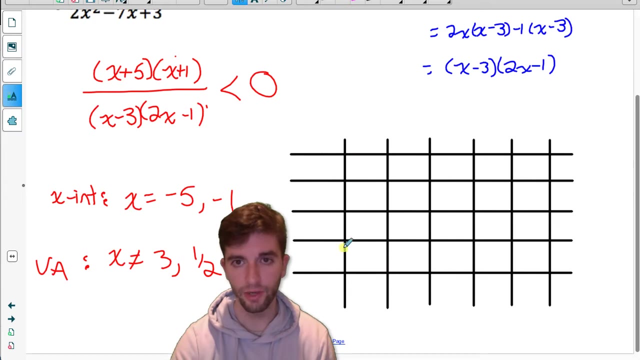 to get that algebraically. We're going to use these as dividing points in our factor table, So let's set up the factor table. Okay, so I very carefully picked how many horizontal and vertical lines to have here. Let me explain how I chose each of. 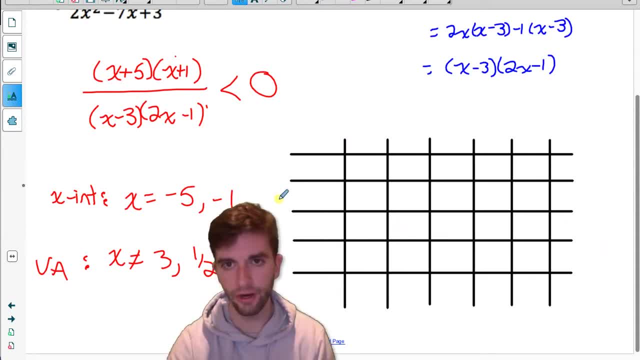 those amounts. So the vertical lines are the dividing points for our intervals. We'll always put negative infinity on the left, positive infinity on the right, And then I needed a vertical line for each of the x-intercepts and for each of the vertical asymptotes. 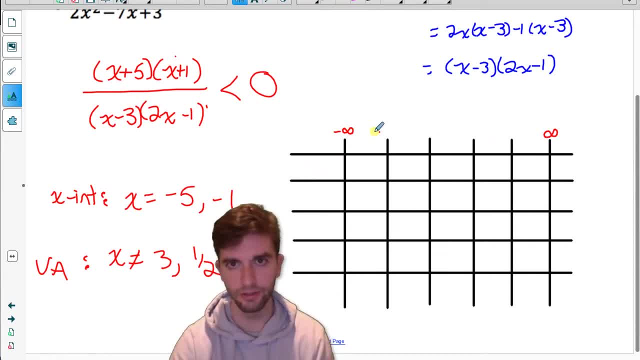 And make sure we write them in ascending order. So negative five, then negative one, then a half, then three. And then how did I decide how many horizontal lines to have? Well, I needed a section for each of these four factors. So I'll put the factor of x plus five here, x plus one here, x minus three. 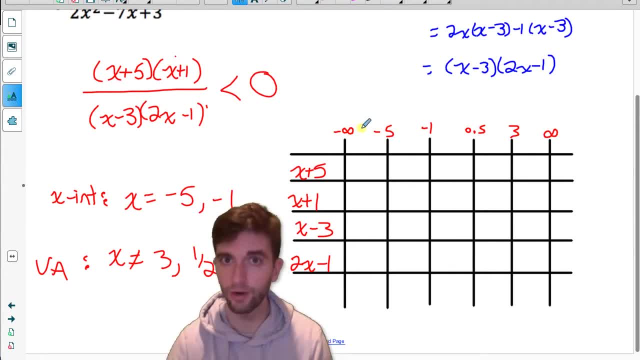 here and two x minus one here. So I need to figure out: within each of these five intervals is the function positive or negative? We're interested in when is it negative, When is it less than zero? And we know at these x-intercepts we're going to have a function that's less than 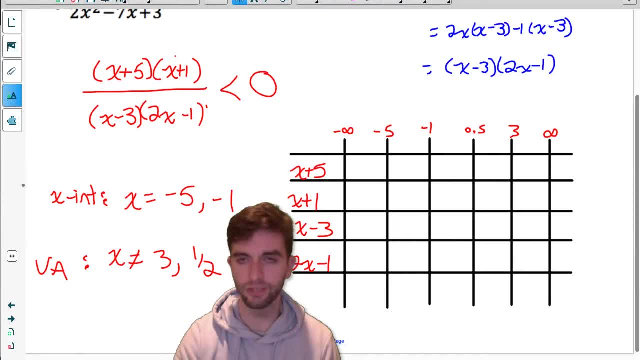 zero. So I need to pick a test point within each interval. So I need to pick a number between negative infinity and negative five. I'll choose negative six, And now I need to see this function at an x value of negative six. Is it positive or negative? So what I'm doing is I'm going to test. 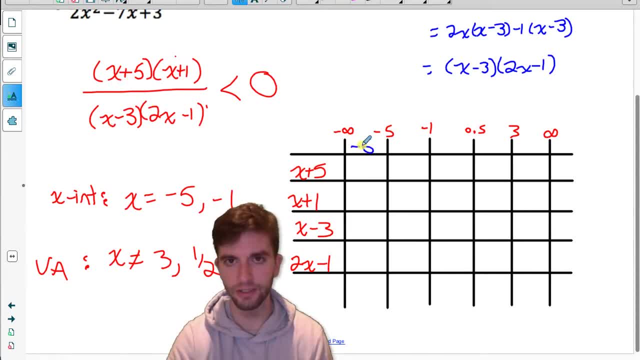 this value in each of those factors separately, In x plus five, I would get negative six plus five, which is negative one. It's a negative result. I don't actually care what the result is, I just care the sign of it, And I'll explain why in a second. 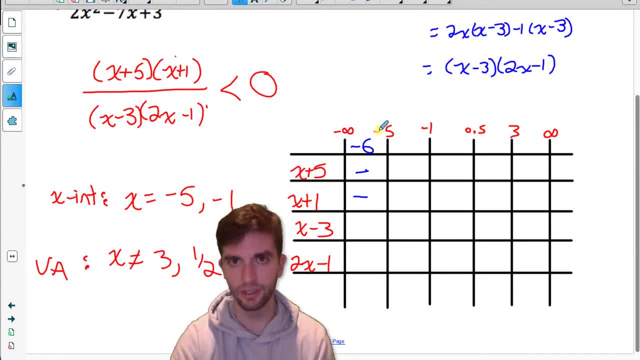 Plug negative six into this factor, I get a negative result. Negative six into this factor: negative result. Negative six into this factor: negative result. So negative six into this whole thing would give me a negative times, a negative which is positive divided by a negative. 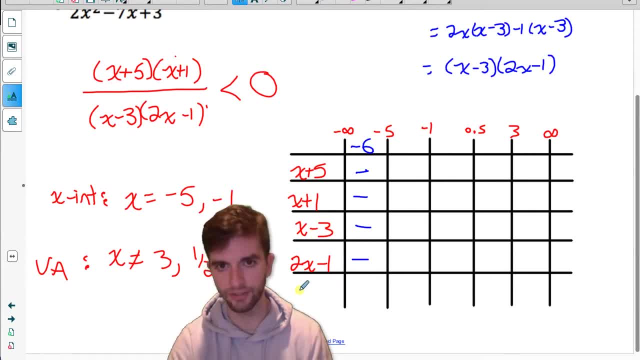 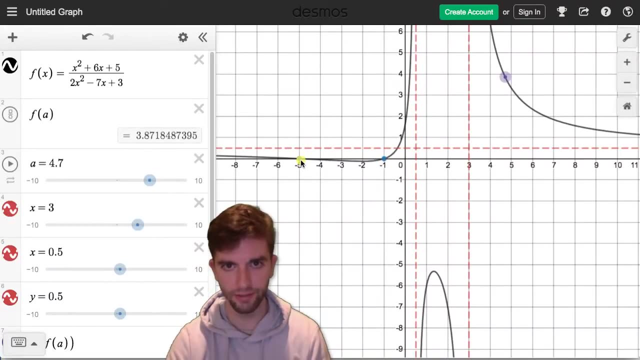 times a negative, which is positive. So I'd have a positive over a positive, So the overall result would be positive. So the function before an x value of negative five is positive And if we look at that graph that I showed you, before an x value of negative five, the function is above the. 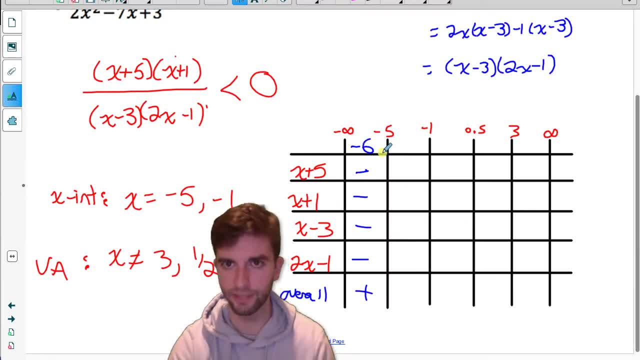 x-axis it's positive. How about between those x-intercepts of negative five and negative one? I'm going to pick a test value of negative two and test it in each of the factors. Negative two plus five is positive three. Negative two plus one is negative one. Negative two minus. 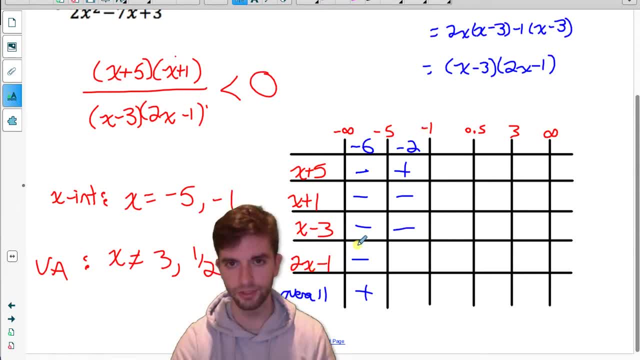 three is negative five And two times negative. two minus one is negative five, So it's negative. So in this factored form version of the polynomial I would have a positive times a negative over a negative times a negative. That would be an overall negative result. An odd number of negative factors. 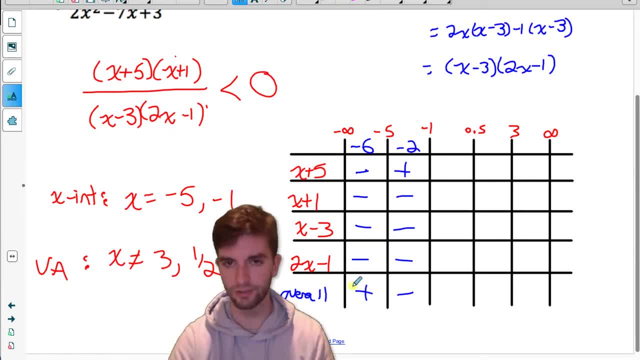 results in a negative result. An even number of negative factors results in a positive result. And now let me, just, Let me just complete these three columns as well, following that same pattern. Okay, now that the table is complete, all we're going to be looking at to answer the question. 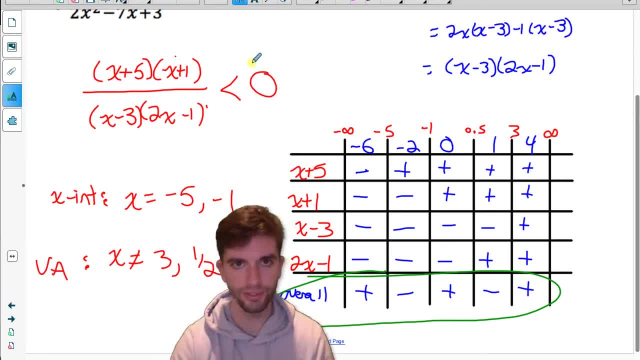 is the bottom row. So the original question says: when is the function less than zero? We know the function will be less than zero whenever the value of this is negative. So in this interval, and again in this interval, So we can answer the. 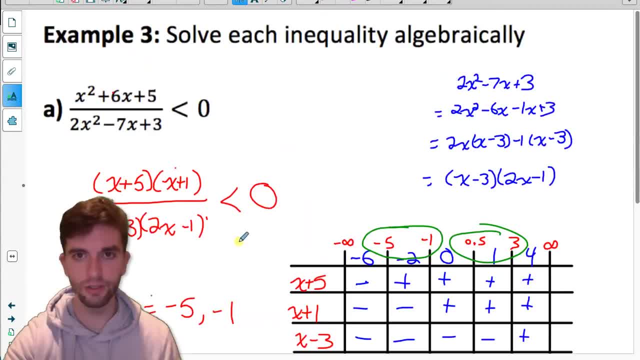 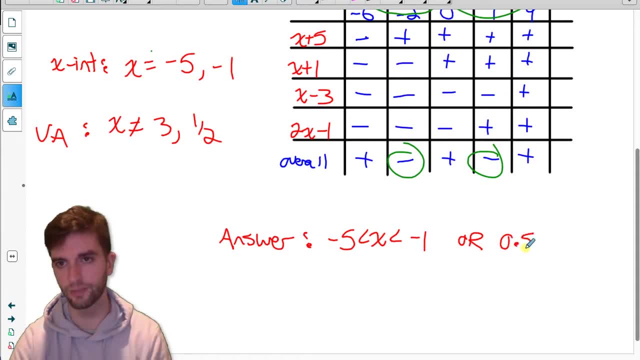 question now. So answer The original. inequality is true if we have an x value between negative five and negative one, or if we have an x value between 0.5 and three. And we can write this in two ways. We could write it like that, with inequality symbols, or we could write it in: 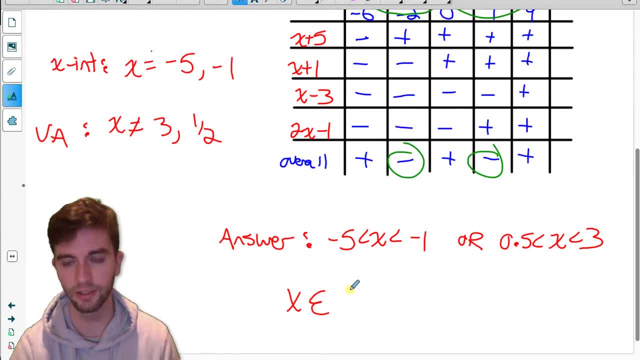 interval notation. So I could say: x is an element Between negative five and negative one, or 0.5 to three. All right, let's try another one. We'll try two more together, and then I'll leave the fourth one for you. 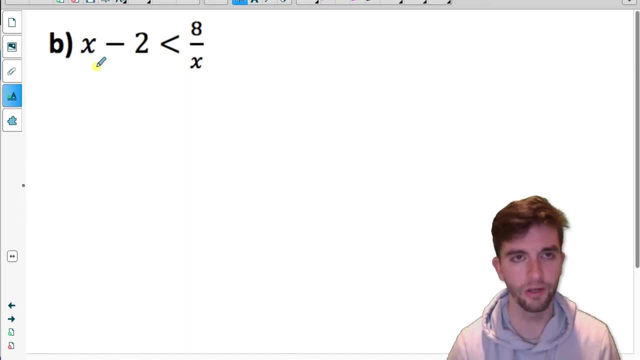 to try on your own, But I'll still show you the solution in this video. So part B: to solve this inequality: resist the temptation to multiply both sides by x, right, Because then we don't know if we have to reverse the inequality or not. We have to split into multiple cases, so don't multiply both. 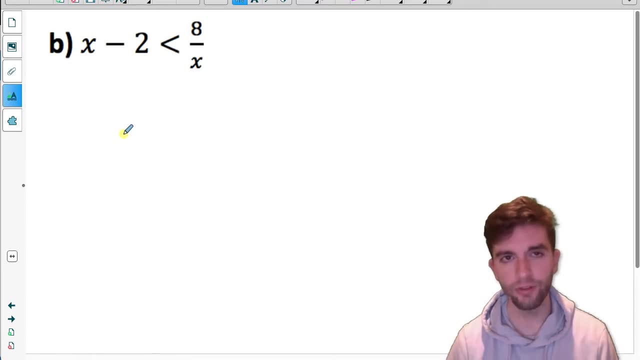 sides by x want to do instead is move all of the terms to one side using inverse operations. So we'll just subtract this term to the left side of this inequality. So I'll have x minus 2 minus 8 over x is less than 0. So all of the terms are now on the left side of this inequality. 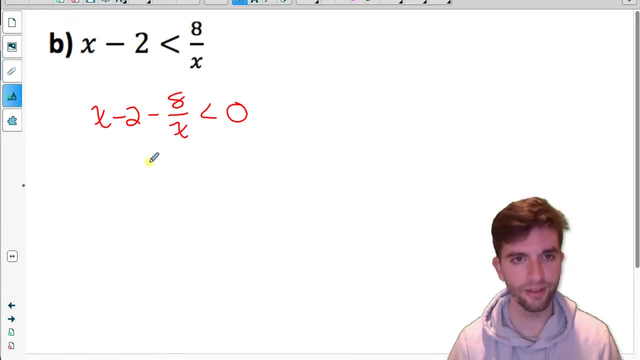 What I need to do now is figure out what the x-intercepts and vertical asymptotes of this are, and the easiest way to do that is to combine all of these as a single fraction. So I need a common denominator. So right now these two terms are both over 1, so a common denominator between these. 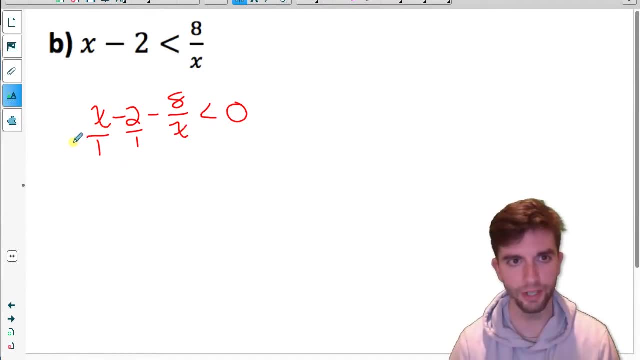 three terms would be x. So I would have to multiply top and bottom of this one by x and top and bottom of this one by x, And then they would all have that same common denominator of x. And you might be saying: well, I thought we weren't allowed to multiply by a variable. Well, x divided by x, that's. 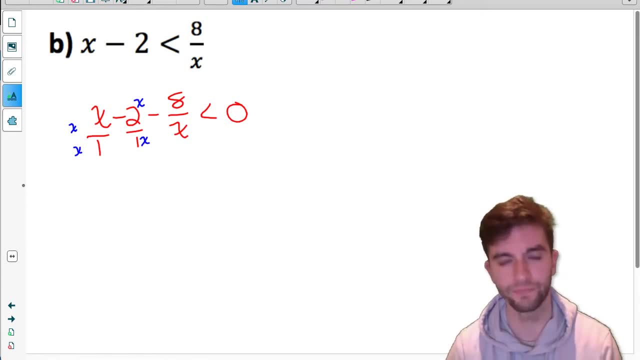 just 1.. We're really just multiplying by 1, so we're allowed to do that. So what I have here x times x is x squared. So I have x squared minus 2x, minus 8, all over that common denominator of x. And we want to know. 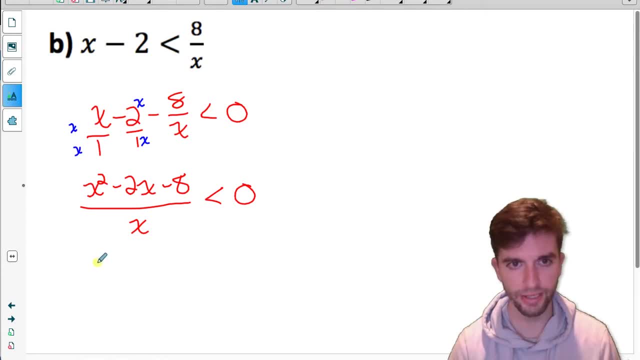 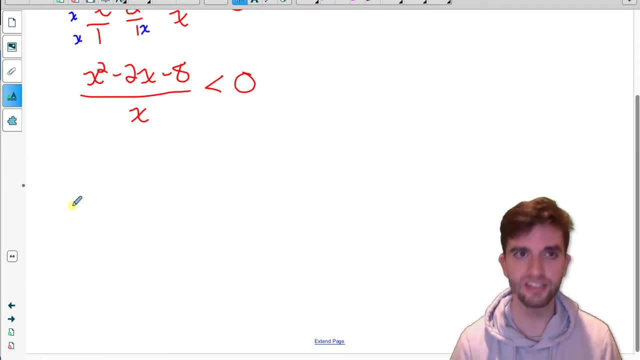 when is this less than 0.. So we're wondering: when is this negative? So what we need to do now is we need to figure out, well, where might it switch from being positive to negative and then test values within those intervals. So where might it switch? It might switch at x-intercepts or 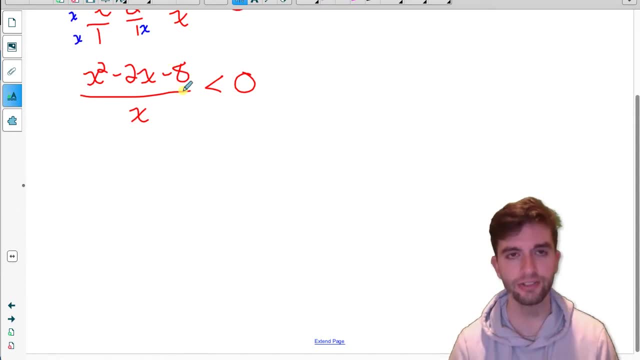 vertical asymptotes. So to find those we should factor this numerator. So the numerator would factor to x minus 4 times x plus 2, because negative 4 and 2 are the numbers that multiply to negative 8 and add to negative 2.. And this is all over x. So we need to list the 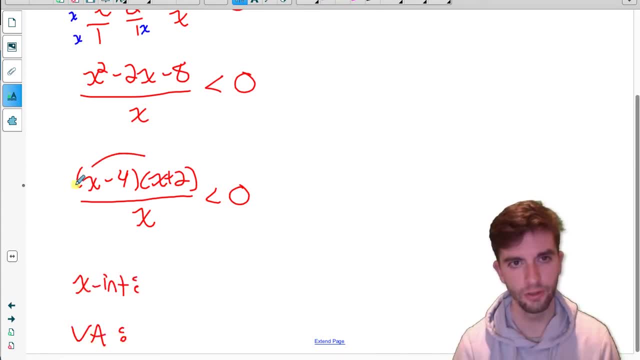 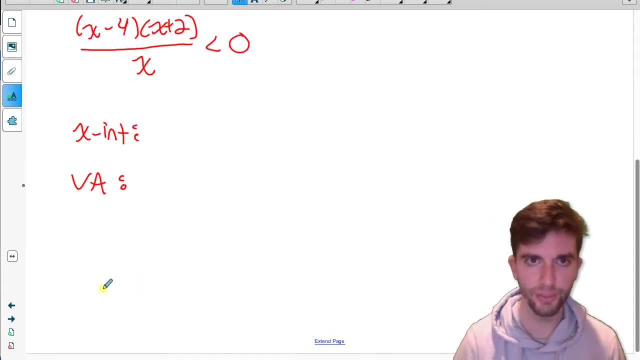 x-intercepts and the vertical asymptotes for this rational function, because if we can figure those out, then we can test values between them and figure out when the function is going to be negative, when it's going to be less than 0. And that's what we're trying to solve. 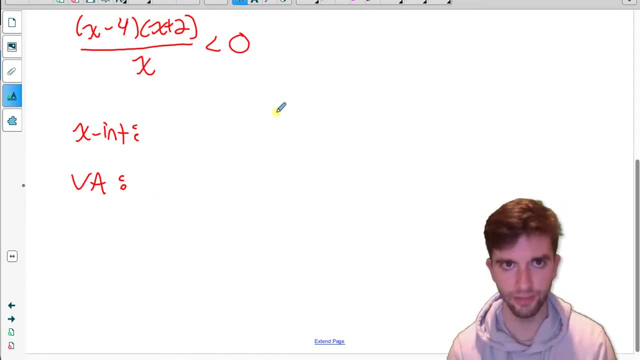 So what are the x-intercepts? Well, x-intercepts have y values of 0. So what would make this whole thing become 0 is whatever would make the numerator become 0. So how could the numerator be 0?? Well, if x was 4 or negative 2.. And vertical asymptotes? Well, vertical asymptotes occur at x. 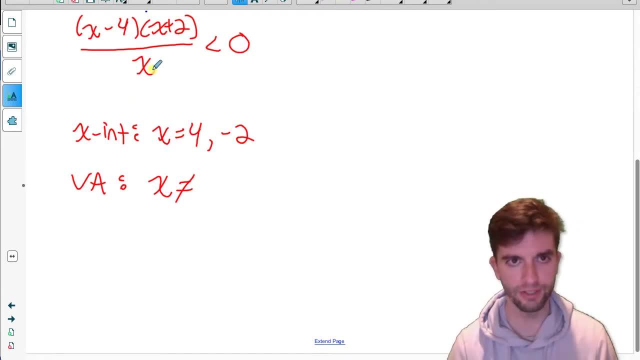 values that would make the denominator become 0. So what would make this denominator become 0? Would be 0. x can't be 0. If x was 0, we'd have negative 8 over 0. That's undefined. So these three values are the dividing points. These three values are the 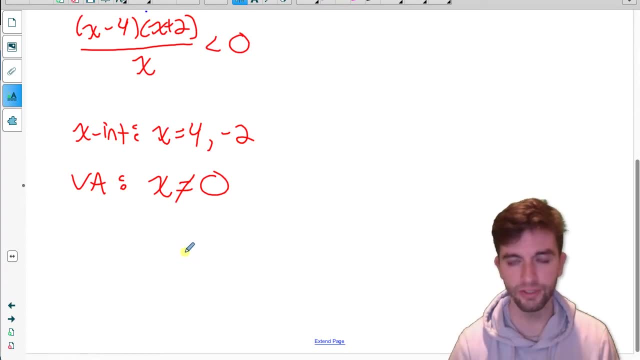 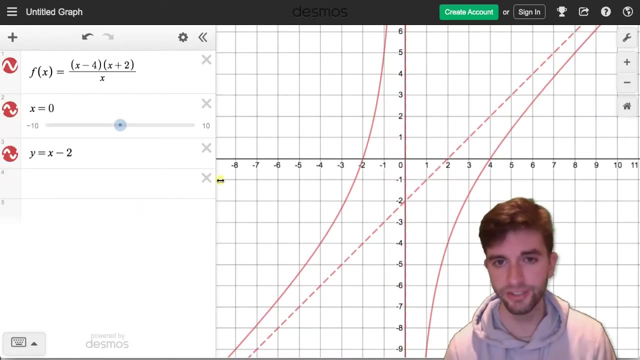 places where the function might switch from being positive to negative or vice versa. Now, we don't have the graph of this function, but let me show it to you, just so you understand what we're talking about. Okay, here's the function. It's an interesting function. It has: 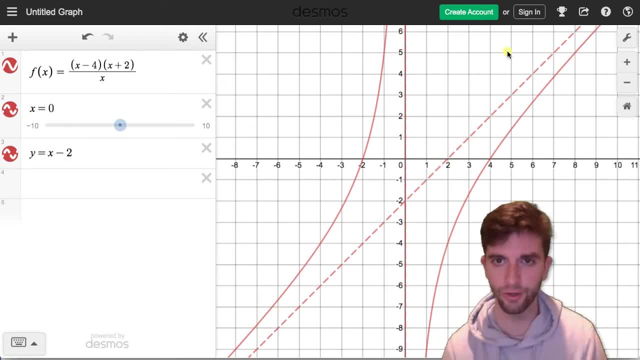 a vertical asymptote and this slant asymptote here also called an oblique asymptote. But we don't really care about being able to generate the graph. I'm just showing you this so we can see why we found the x-intercepts and vertical asymptotes. 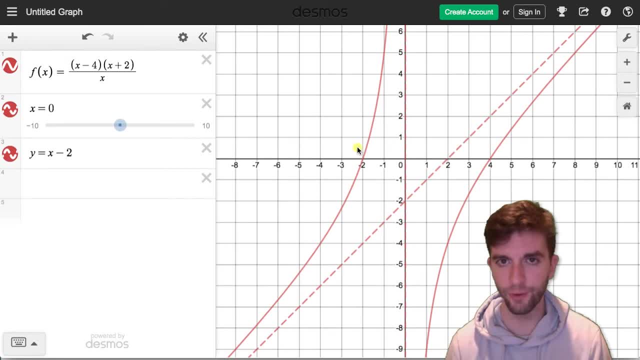 Notice the function is negative before the x-intercept of negative 2 and then positive after, So that x-intercept is a place where it switches signs And then it's positive forever. it appears until it gets to the other side of the vertical asymptote. Then the function 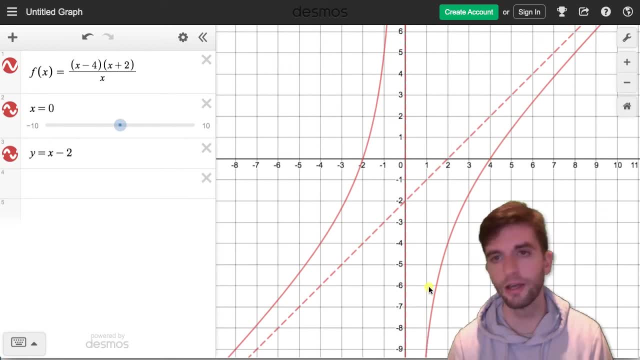 reappears down here with negative y values, And then it switches from negative y values to positive y values after this x-intercept- right there. So those two x-intercepts and this vertical asymptote are the places where the function can switch signs. So we just need to test values. 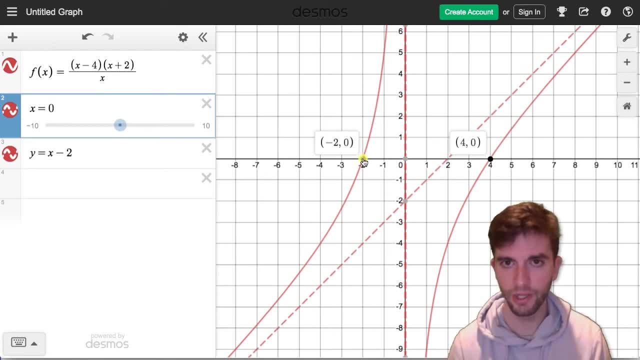 within each interval: The interval before negative 2, between negative 2 and 0, between 0 and 4, and between 4 and infinity. We test where the function is in each of those intervals and then we can figure out the answer to our inequality, which wants to know: when is it less than 0. So 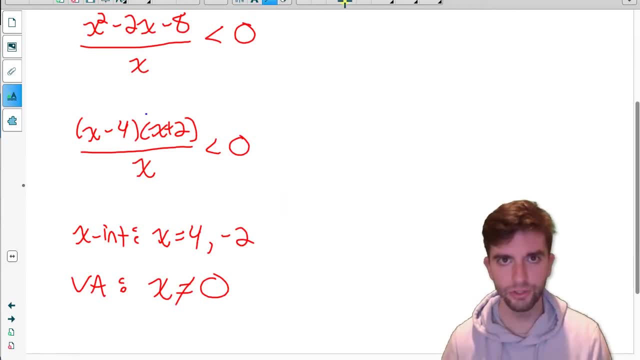 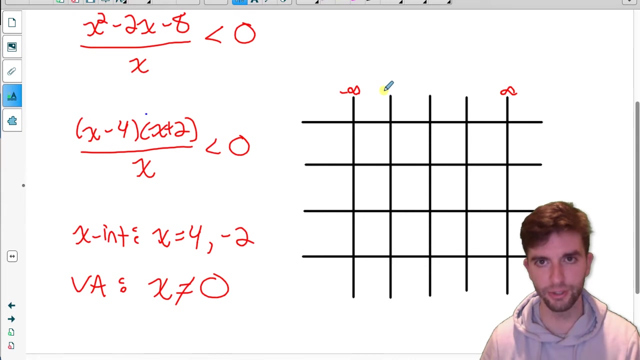 when is it negative? So we'll make our factor table, So we'll draw those horizontal and vertical lines again. I chose five vertical lines because I need one for negative infinity, positive infinity, and then each of these three values, making sure to put them in ascending order. So negative, 2,, 0,, 4.. And 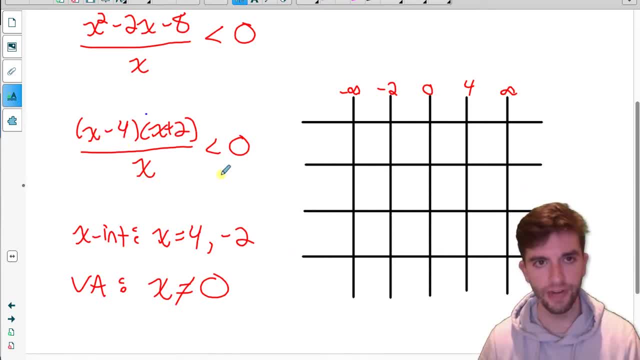 then I also need a row for each of the factors. So I need a row for x minus 4, for x plus 2, and for x. At the very bottom. I'll state the overall sign of this rational function here. So I need to now. 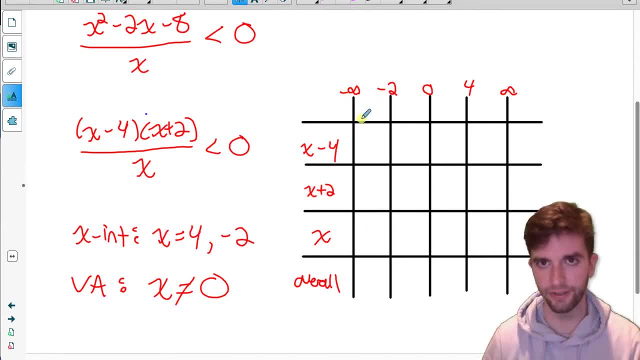 plug in negative 3 within each of these intervals. So I'll pick a test point between negative infinity and negative 2, a test point in this interval, in this interval and in this interval. And these test points, remember, these are x values we're choosing. We're choosing x values to plug into this, to see. 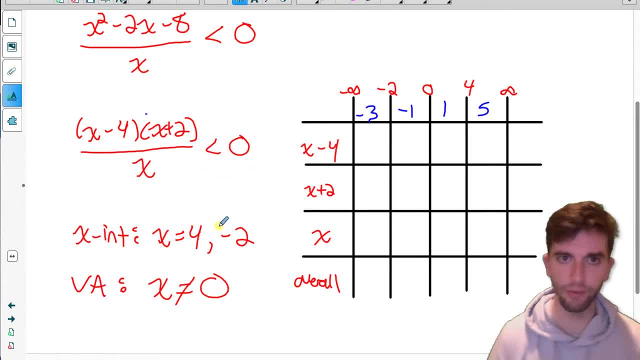 if it's positive or negative. If it's negative, well, a negative number is less than 0, so that will be an answer to the inequality. So, instead of plugging into the whole thing and evaluating, I'm just going to plug it into each factor one by one. So plug in negative 3 to x minus 4, and then I'm 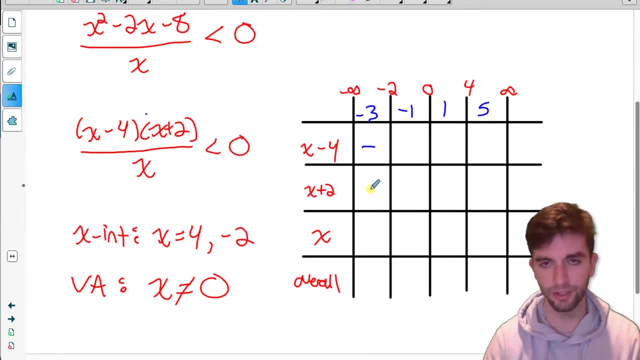 going to plug in x minus 4. That's a negative result. Negative 3 into x plus 2.. Negative 3 plus 2 is negative 1, so that's a negative result. And negative 3 in for x is of course negative. So I figured. 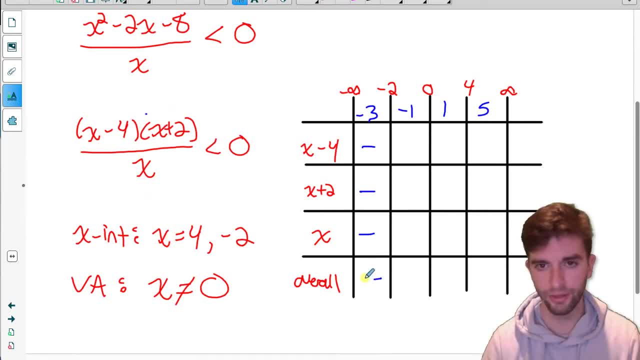 out, I would have negative times. negative divided by negative, That's a negative result. Odd number of negative factors is a negative result. So let's follow that same process for these three intervals. Okay, now that we've done that, let's go ahead and plug in negative 3.. 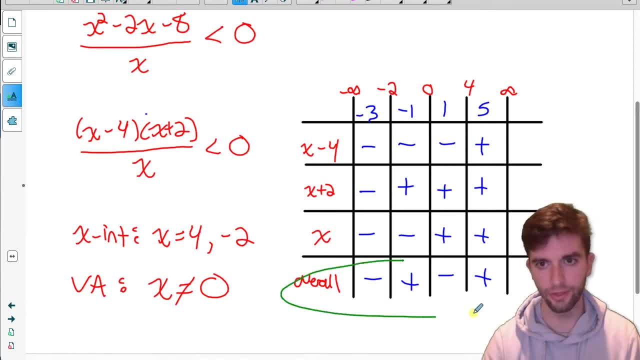 Now that we have the factor table complete, all we have to do is look at the bottom row and look for when is it negative, because our inequality is asking: when is this less than 0.. So it's less than 0 whenever it's negative. It's negative in that interval and in this interval. So I could. 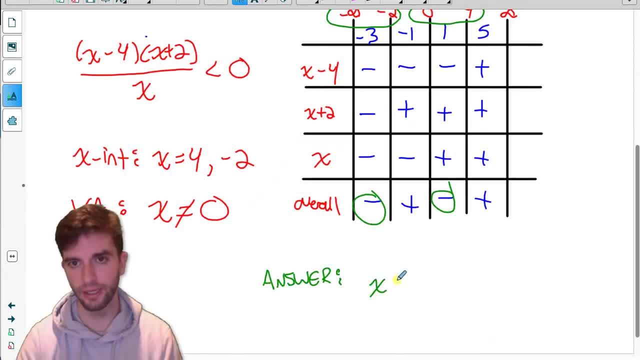 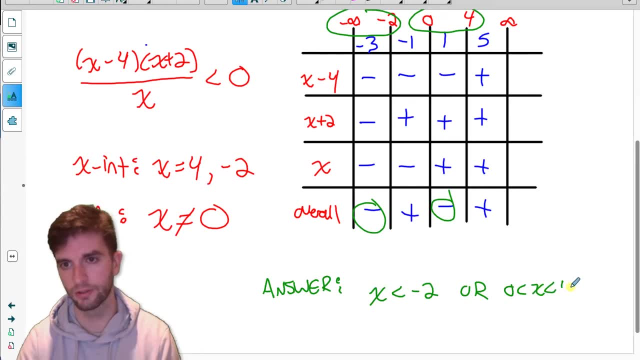 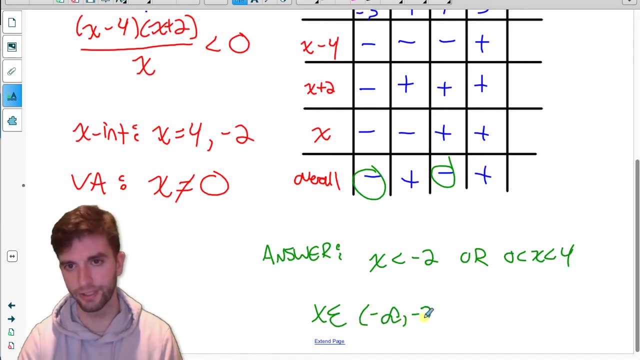 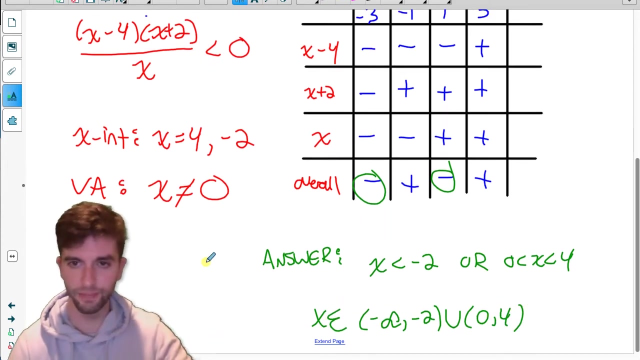 write that in two ways: As inequalities. I could say x less than negative 2, or between 0 and 4, or I could write it in interval notation. I could say x is an element between negative infinity and negative 2, or between 0 and 4.. Either way of expressing your answer is fine. Let's just compare. 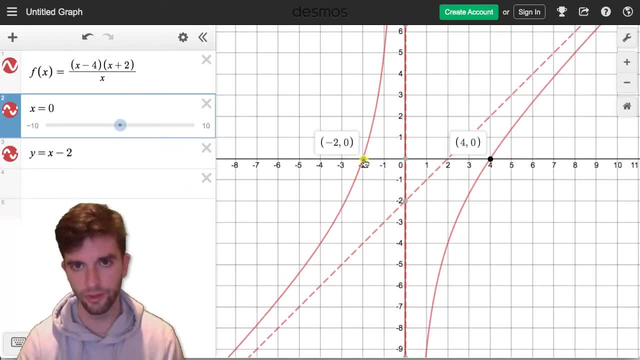 that to the graph and make sure we found the right intervals. Notice the function is less than 0 when x is less than negative 2, and again between 0 and 4.. The function is down here. It's negative, So we. 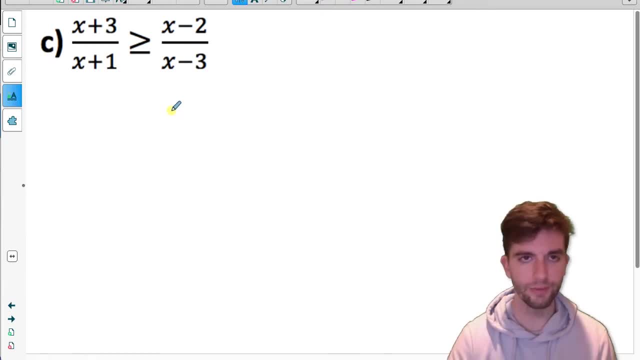 found the correct two intervals. So let's look at the graph. So we found the correct two intervals. Part c: once again, resist the temptation to cross multiply. We don't want to be multiplying both sides by any variables, So instead we're just going to move this whole term to this side of. 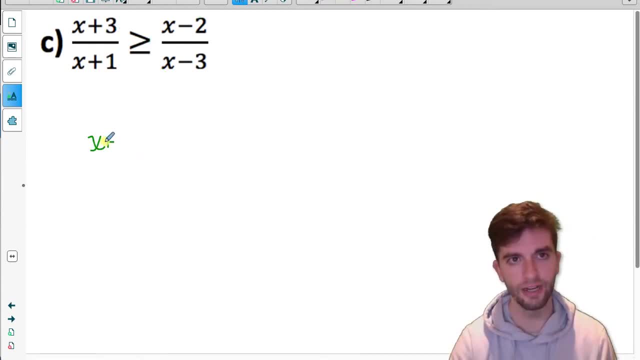 the inequality. So we're going to subtract it over. So I have x plus 3 over x plus 1. minus x minus 2 over x minus 3 is greater than or equal to 0. Well, this is the first time that we have an. 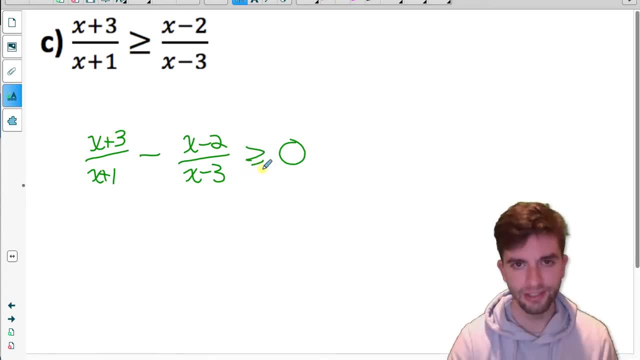 equal sign underneath our inequality. The only time we really have to consider that is when we're expressing our final answer, and I'll talk more about that when we get there, But for now, let's follow the same steps we did for a and b. 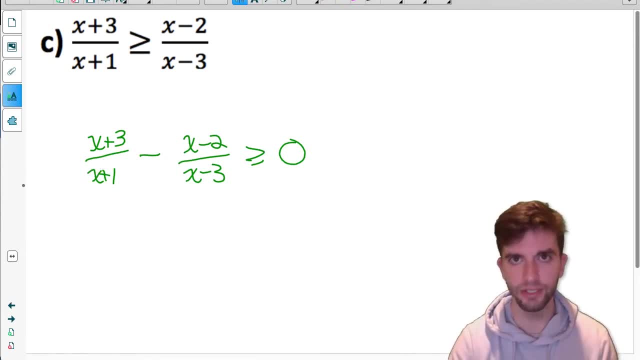 Now that we have everything on one side, let's get a common denominator. So I need to multiply this one top and bottom by x minus 3, and this one top and bottom by x plus 1.. Now you should notice they both have a common denominator: x minus 3 times x plus 1.. So I can write this as: 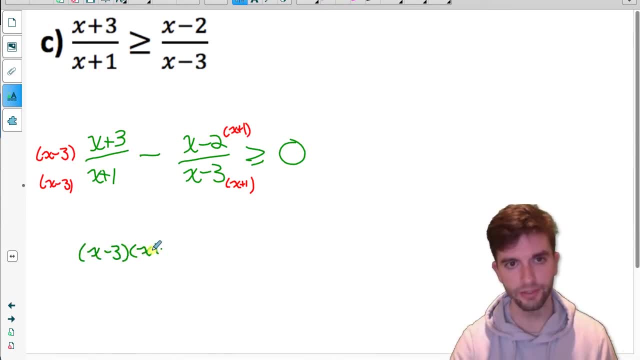 a single fraction: x minus 3 times x plus 3.. Minus this product: x minus 2 times x plus 1.. All over that common denominator, x minus 3 times x plus 1.. And we want to know when is this greater than or equal to 0.. To figure out when is it greater than or equal to 0,. 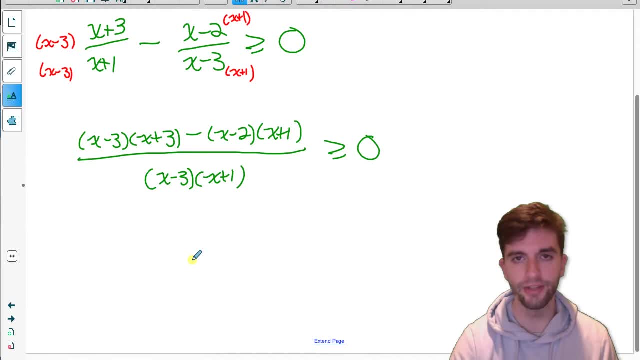 I'm going to have to find the x-intercepts and vertical asymptotes and then test points within the intervals Before I can find the x-intercepts. this up here is not in fully factored form. There's this minus sign here. 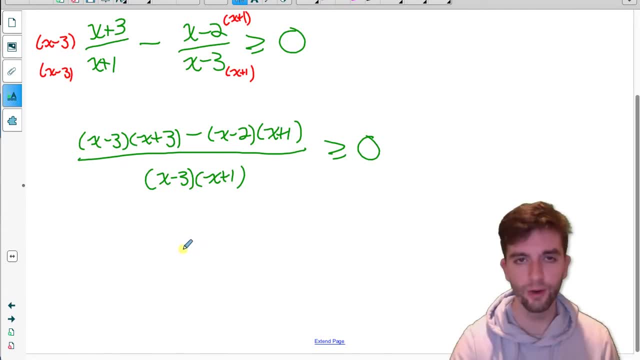 So what I'm going to have to do is expand this and collect some like terms and hopefully, through that process, be able to find what the x-intercepts are. So this is a difference of squares. that would be x squared minus 9. Minus. make sure you put this product in brackets so that we know we have. 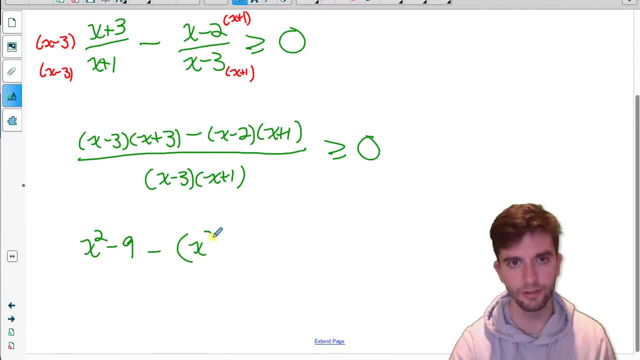 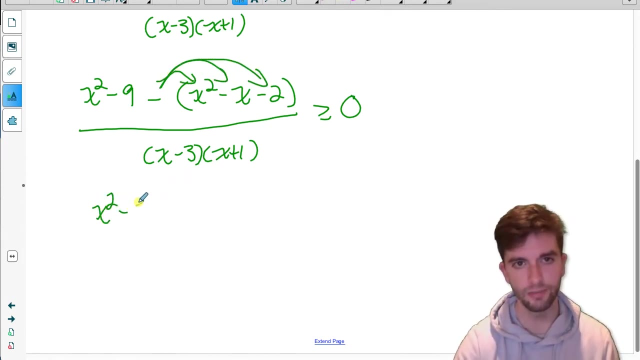 to subtract the whole product, So this product would be x squared plus x minus 2x, that's minus x minus 2.. And this is all over that common denominator. Now I can subtract all three of these terms, So I have x squared minus 9, minus x squared plus x plus 2.. To collect: 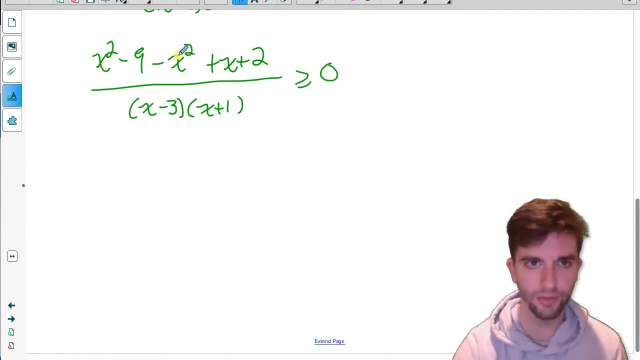 like terms in the numerator: x squared minus x squared. those cancel out, that's 0.. And I have an x and a negative 9 plus 2, that's negative 7.. Ok, so now it should be obvious what the x-intercepts and vertical asymptotes are. X-intercepts are x values that make the 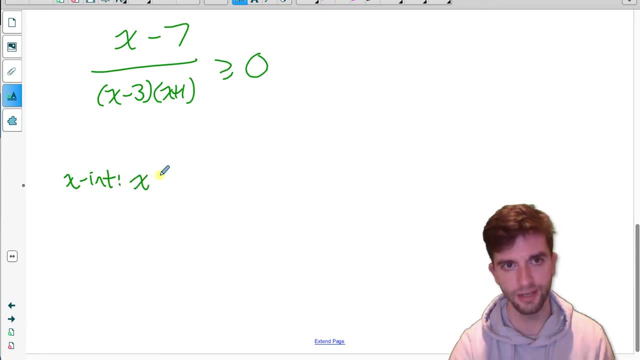 numerator become 0, so the only x-intercept is at an x value of 7.. And the vertical asymptotes: asymptotes are x values that make the denominator be 0. So x can't be 3 or negative 1. Either of. 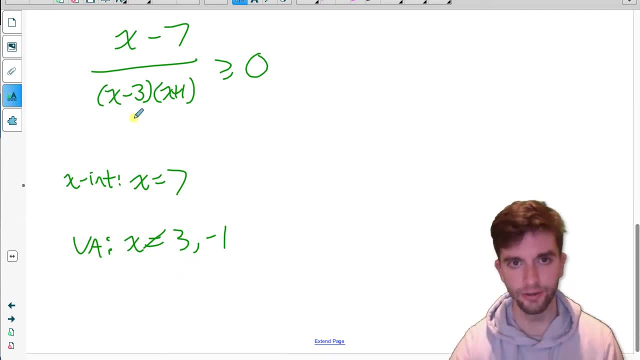 those would make the denominator 0, making this whole rational function undefined. So these three values are the places where the function might switch from being positive to negative, So we'll use those as dividing points and test x values within each of the intervals In this question. 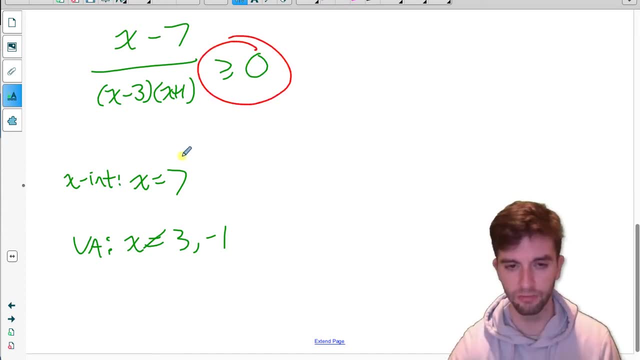 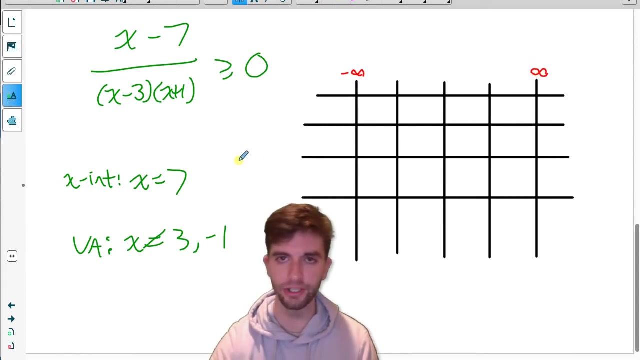 we're interested in. when is the function greater than or equal to 0. So when is it 0 or positive? So let's set up our factor table. So, once again, far left is negative infinity, far right is positive infinity, and then between those, 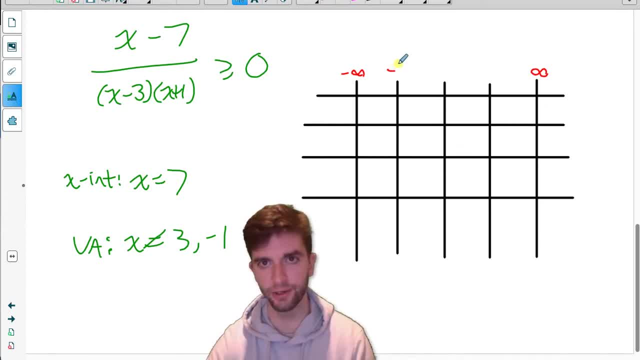 two. I need each of these three values in ascending order: negative: 1,, 3,, 7.. And then I need a row for each of the factors: x minus 7,, x minus 3, and x plus 1.. And now I get to choose my function. 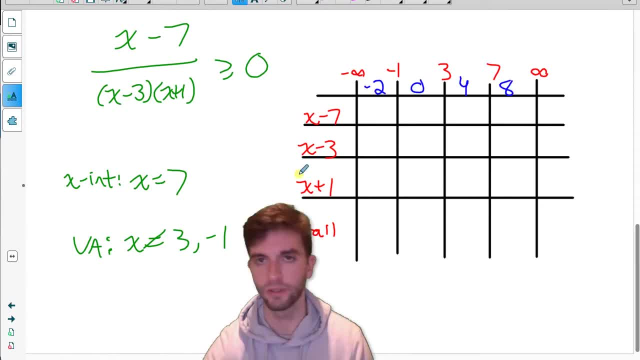 I get to choose my test values for x within each interval. Your test values don't have to be the same as mine. Just pick any number between negative 1 and 3 and put it there. I just chose 0 because I thought that was an easy number to work with. Okay, now let's test each of these. 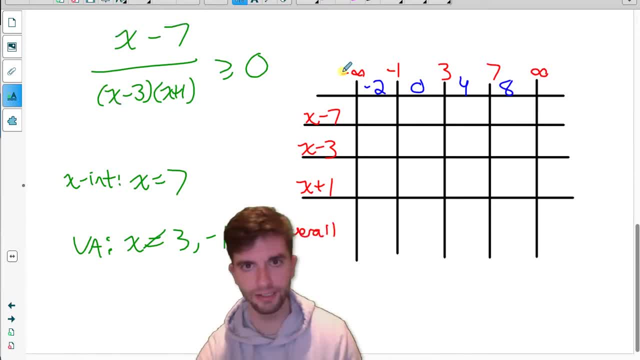 numbers in this whole rational function, by plugging into each factor one at a time, and seeing if we get a positive or negative result. Negative 2 minus 7 is negative 9,. negative 2 minus 3 is negative 5, and negative 2 plus 1 is negative 9.. So we get a positive or negative result. 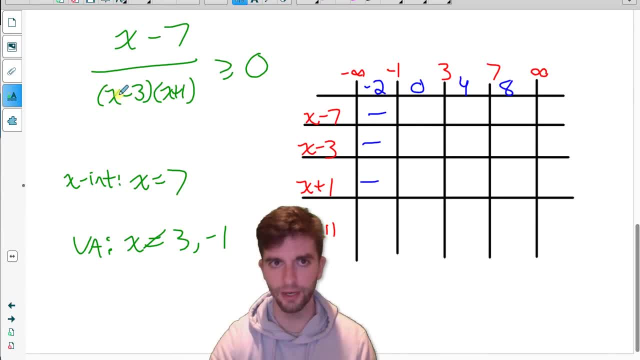 And then the remaining 1 minus 7 is negative 1.. So we have a negative divided by a negative times a negative and odd number of negative factors is an overall negative value. So the interval between negative infinity and negative 1 is not a solution to the inequality. The 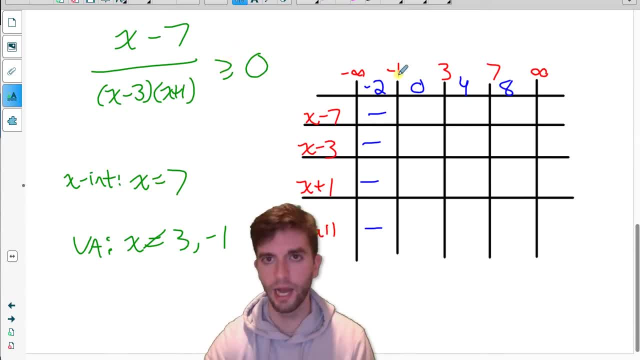 function is not greater than or equal to zero there. It's less than zero there. How about in this interval, negative 1 to 3.. Let's plug 0 in for each of them and I get a positive result. Good, I found one interval that is a solution to my inequality. I now know it's. 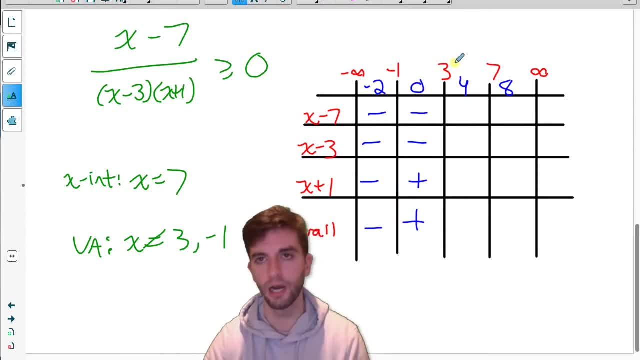 greater than zero, between negative one and three. How about this interval? So this interval is not a solution. it's negative there. And how about this interval? This interval is also a solution because it's positive there. right, We're interested in when is it greater than or equal? 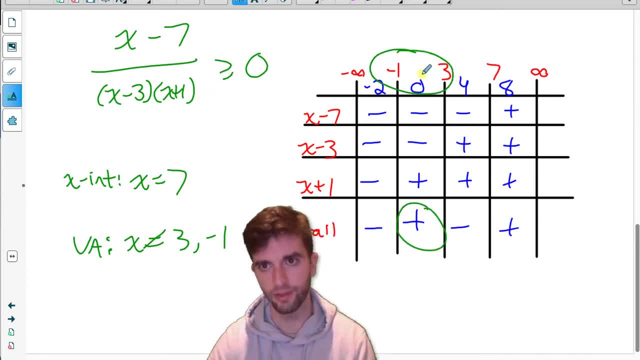 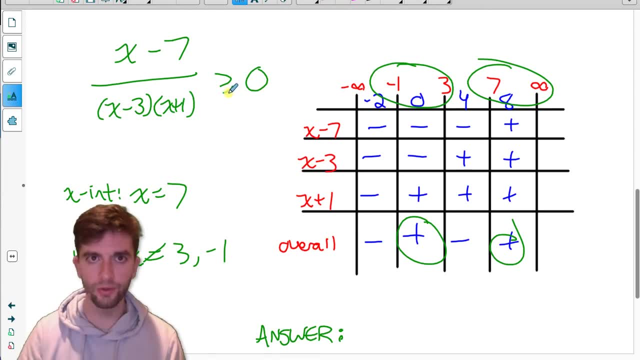 to zero. So we're interested in when is it positive? it's positive there And there. So when we describe our answer, we have to be careful that we include not only the intervals where the function is greater than zero, but also the places where it's equal to zero. So we have to make sure. 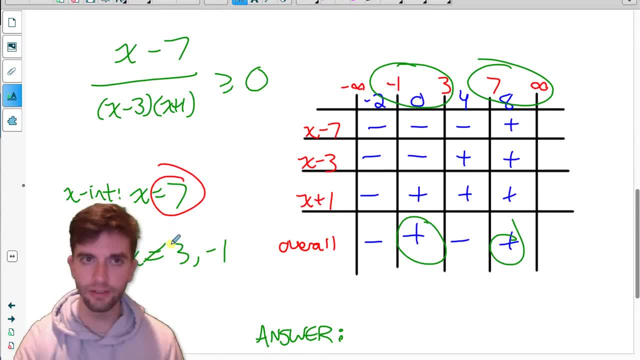 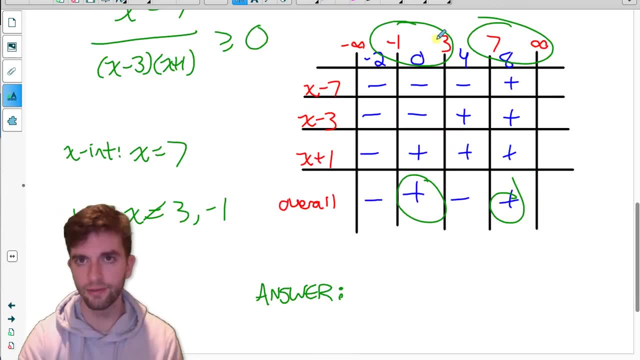 that we include seven in the answer, because at seven this whole thing is zero And we want to include that in our answer. So let's watch how we do that. So between negative one and three the function is positive. So in our answer we'll say x is between negative one and three. 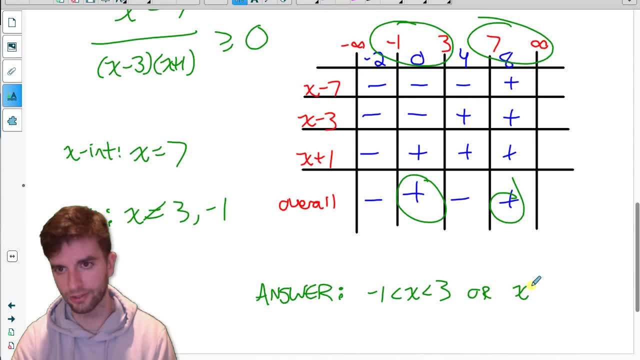 And when x is greater than seven. so we'll say or x is greater than zero Seven. But I need to include seven in my answer because that is a place where the function actually equals zero. So how do I include it? I put an equal sign under there as well. it says: 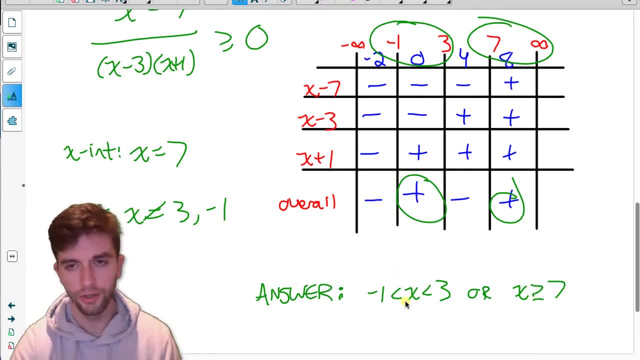 when x is greater than or equal to seven. no equal sign under these two, because at negative one and three the function is undefined. So that's of course not an answer to when it's greater than or equal to zero. So how could I write it? in bracket notation I would say: x is an element of 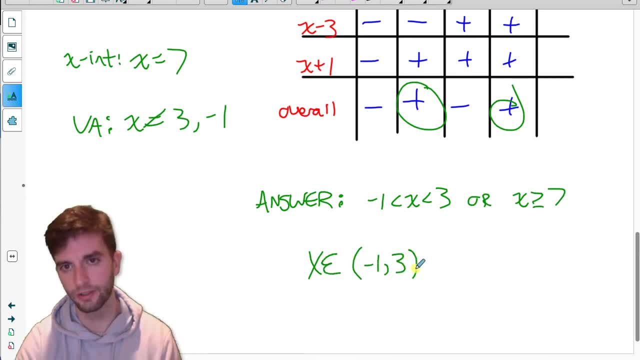 negative one to three To three or seven to infinity, And I was very careful to put a square bracket at seven to make sure that shows that it's included in the answer. round brackets at negative one, three and infinity, because those are not included in the answer. Okay, we've done three examples together. 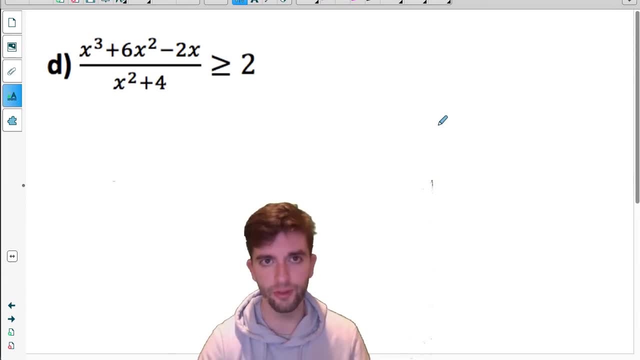 I think it'd be a good idea now if you were to pause the video and try this one on your own And then, after you give it a try, unpause and see how you did. I'll show you how to do that. So the solution Now- this one is probably the most difficult of the four, So don't get discouraged. 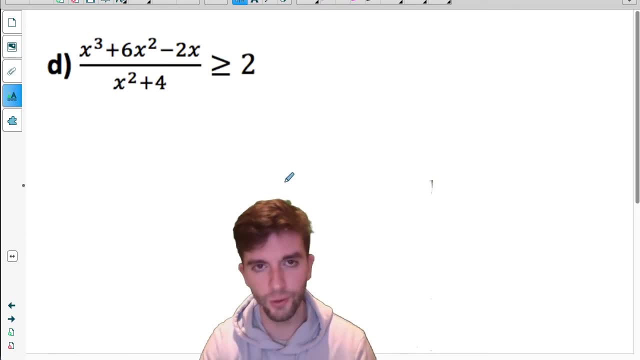 if it takes you a little bit of time or if you don't get it right, Just follow along after and fill in the proper solution. So pause now and give it a try. Okay, so here's the solution. just follow along. 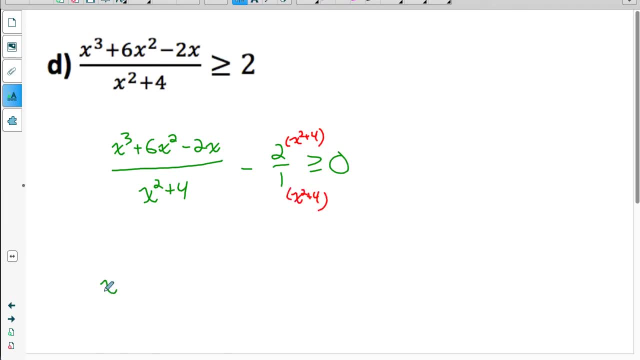 As I said, I'm gonna turn on the volume, I'm gonna change the volume and I'll just always keep on FM that way, because I don't want it to be too loud And it's gonna go back and I'll just. 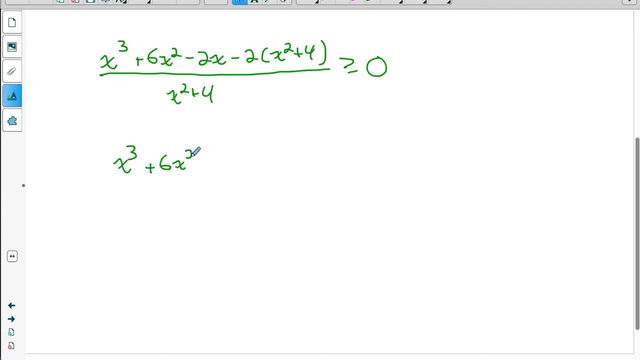 keep on FM. that way- Like, for example, when you're on the right side of the screen- you'll just keep on using the volume. Just think about it. if you want to update the volume or you want to make the volume larger, you can go back and change the volume and it's gonna automatically stay.